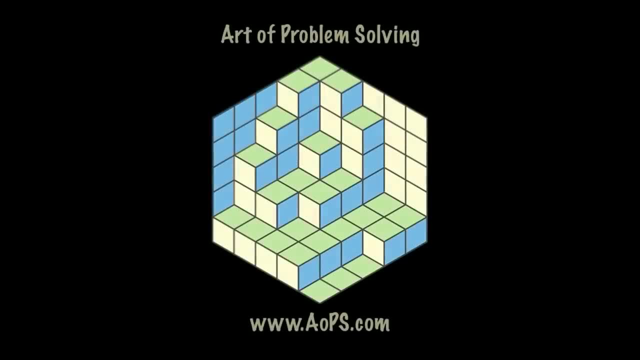 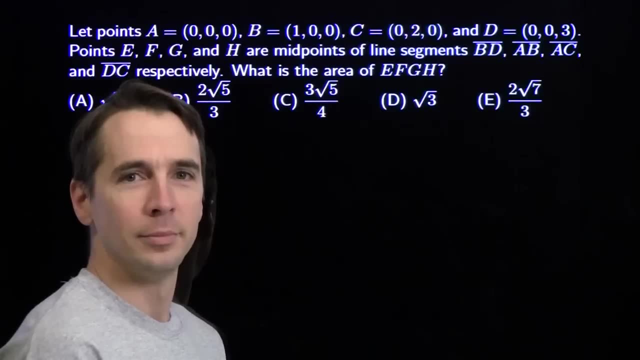 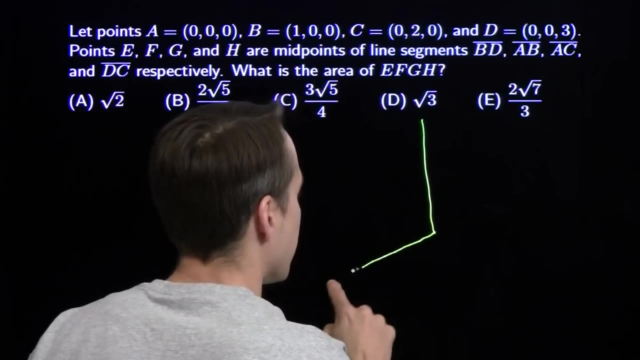 We've got a little 3D geometry here. We'll start off with a quick sketch. First, the coordinate axes: We've got our z-axis, our x-axis and our y-axis- X, y and z. Now 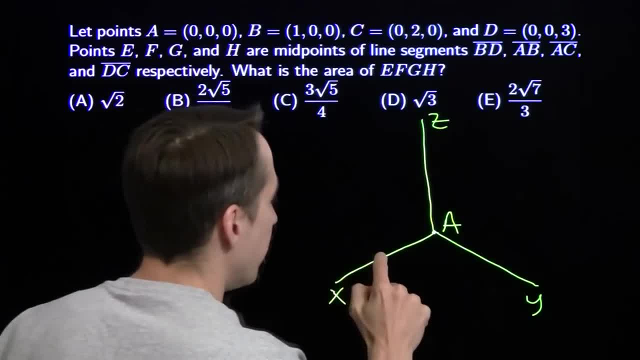 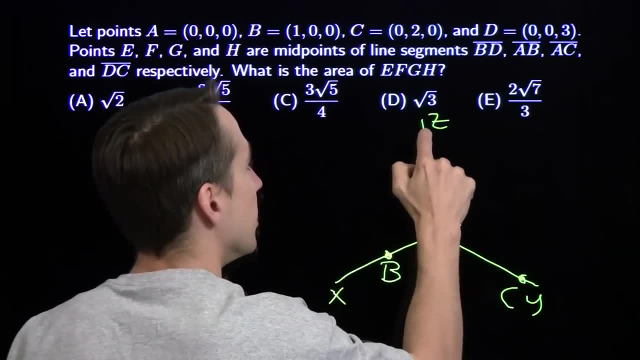 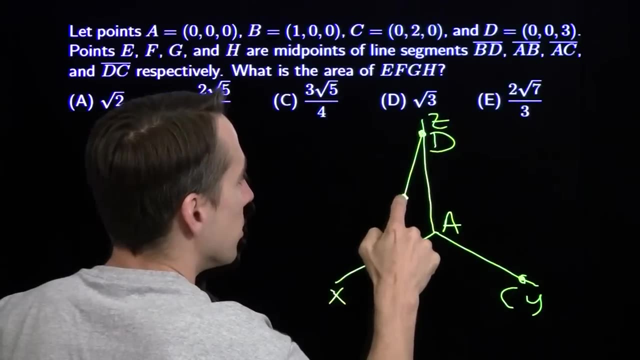 A is the origin, B is out here on the x-axis, C is over here on the y-axis And D is up on the z-axis. Now E is the midpoint of BD. E is the midpoint of BD. F is the midpoint. 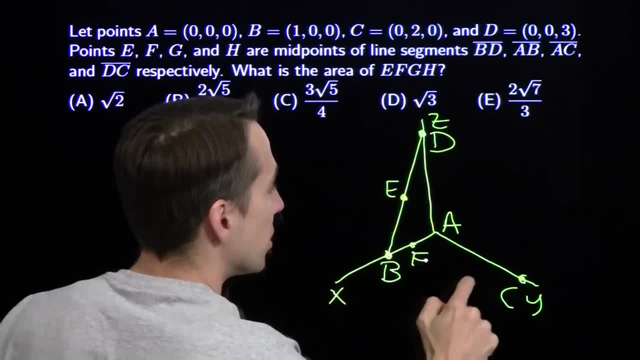 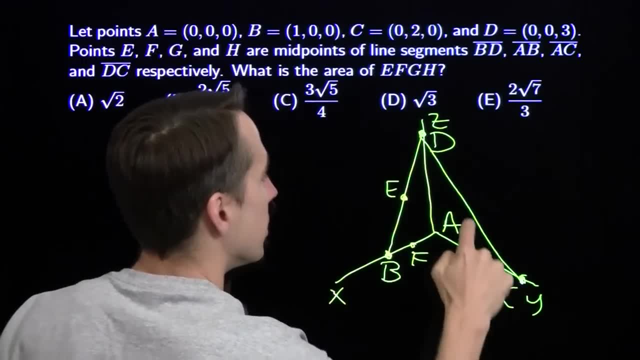 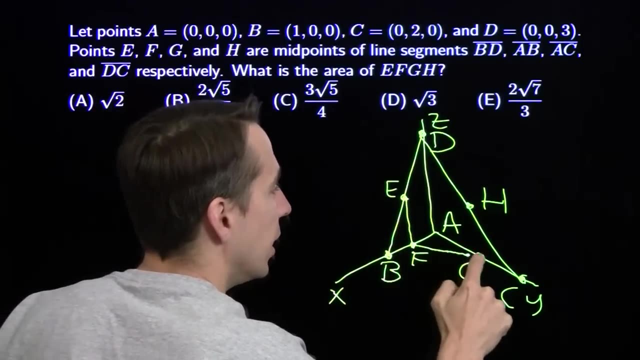 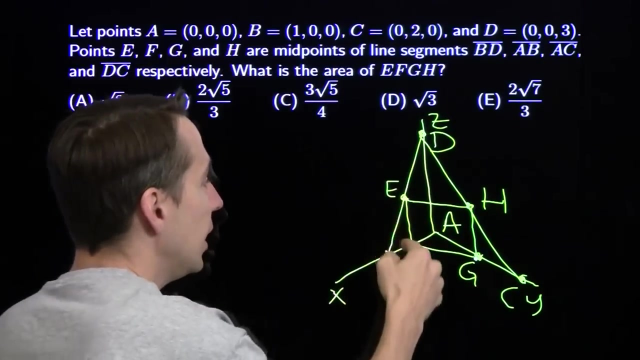 of AB. G is the midpoint of AC And finally H. H is the midpoint of DC And we need to find the area of this quadrilateral right here: EFGH. Now we'll start by focusing on the fact that these are midpoints. E and F are 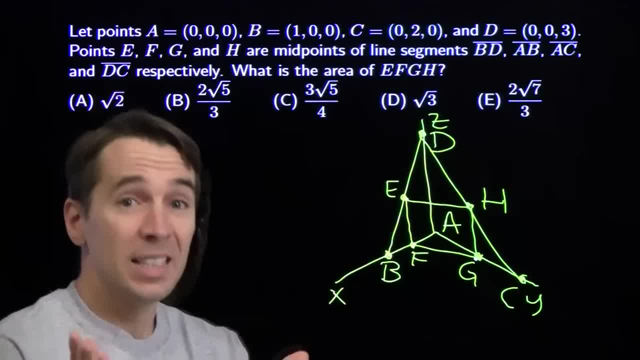 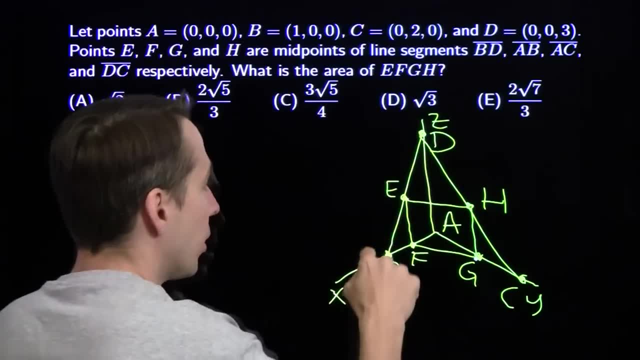 midpoints of sides DB and AB. This gives us a little side-angle-side similarity We've got: EB is half of DB, FB is half of AB And of course angle EBF equals angle DBA. So EFGH is half of DB, FB is half of AB And of course angle EBF equals angle DBA. So EFGH is half of DB And of course, angle EBF equals angle DBA. So EFGH is half of DB And of course angle EBF equals angle DBA. So EFGH is half of DB And, of course, angle EBF. 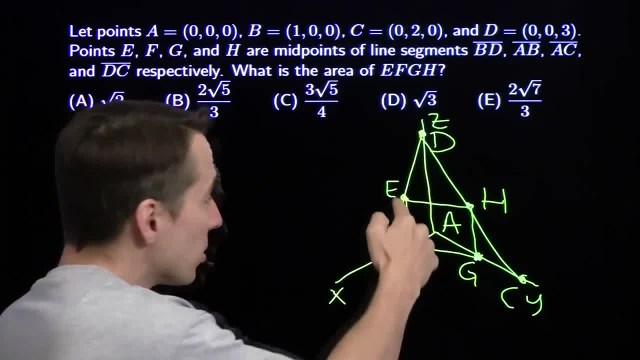 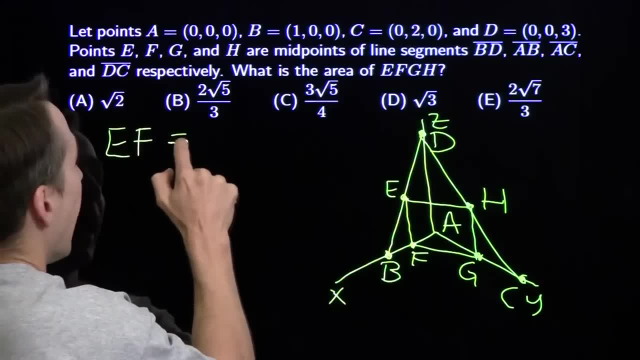 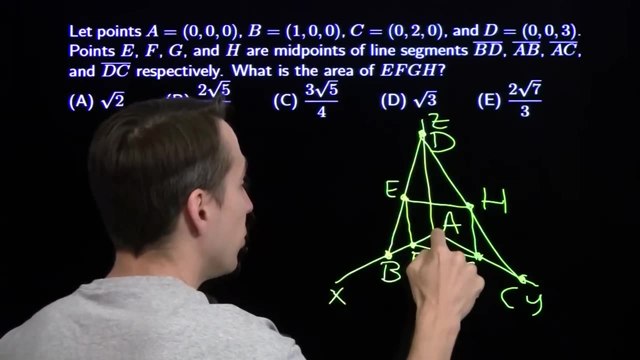 is similar to DBA. EB is half of DB, So EF is half of AD. That tells us that EF is three halves, because we're given that AD is three. Even better, we found out that angle EFB is equal to angle DAB. That means angle EFB is 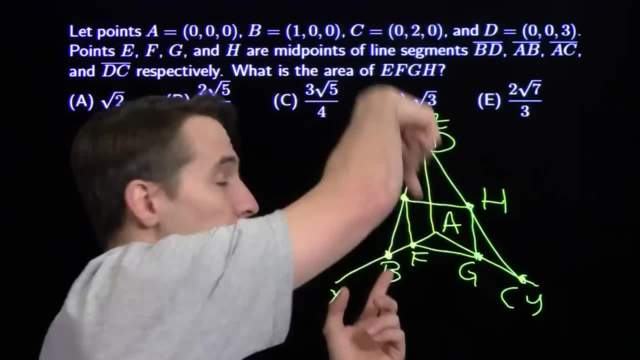 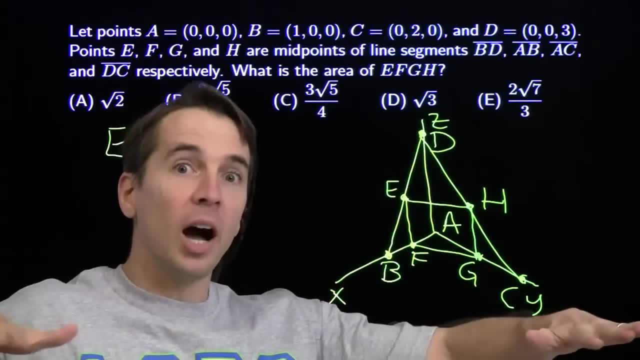 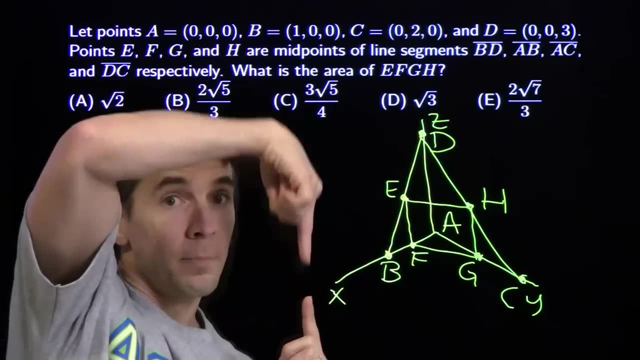 a right angle And it tells us EF is parallel to AD. EF is parallel to the z-axis. The z-axis is perpendicular to the entire xy-plane. You've got the xy-plane here, You've got the z-axis pointing straight down at it. So EF is parallel to the z-axis. That means it's perpendicular. 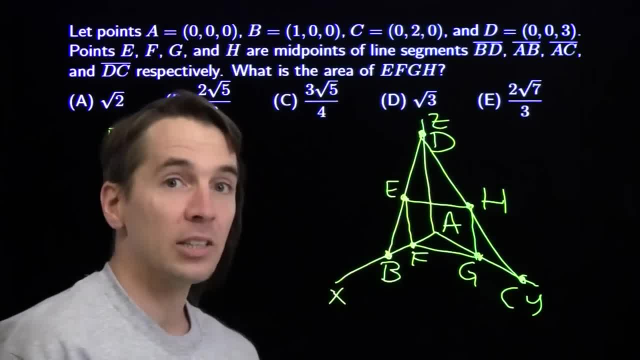 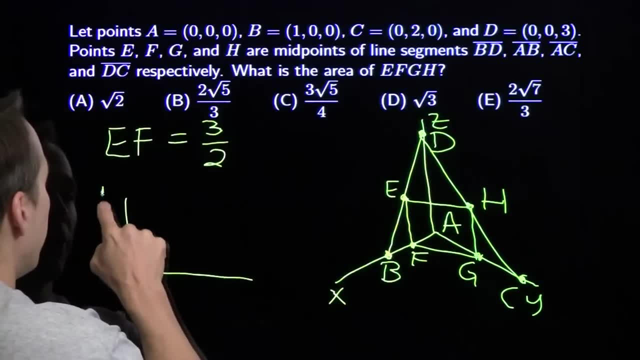 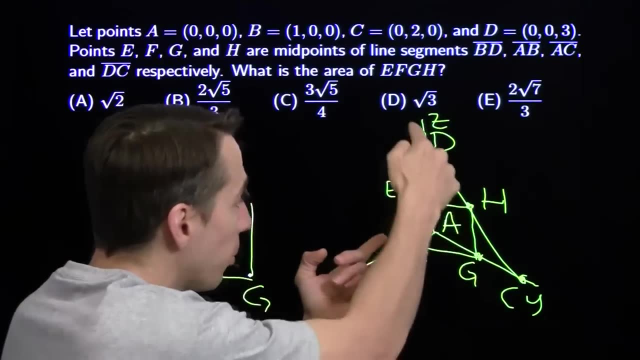 to the entire xy-plane. That means EF is perpendicular to FG. So now we know that our quadrilateral looks a little something like this: We've got EF over here And we know that it's perpendicular to FG. Now we do the same game over here. H and G are midpoints of DC and FG And we